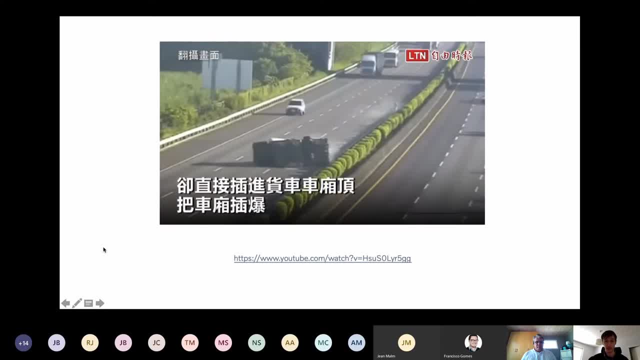 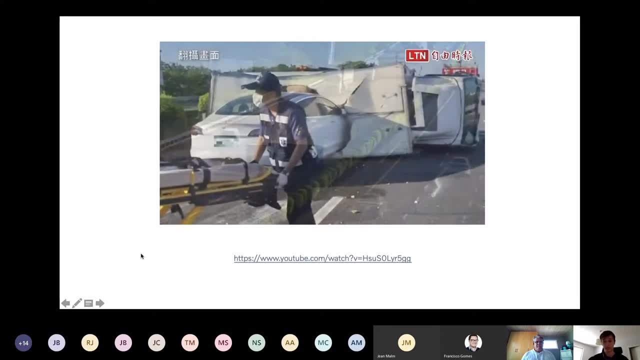 Because it's obviously that a truck, a white truck, lying in the middle of a highway is an anomaly, And also the roof was white color And it seems like the Object detection algorithm messed it up with the sky or something. So yeah, this is like a background of why we need anomaly detection. 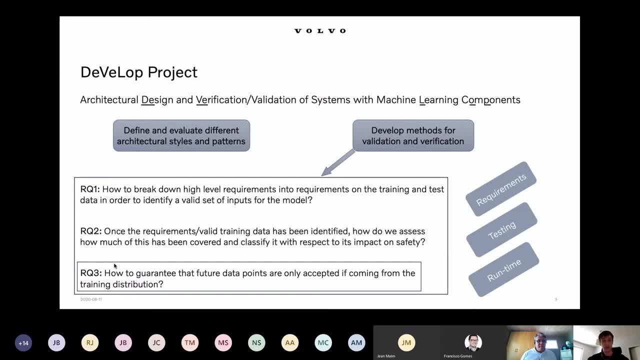 Next slide. I want to talk a little bit about my our general topic, which is developed project. We are working on the architectural design and verification and validation of systems and machine learning components, And it basically consists of two different parts, which are: architectural part. 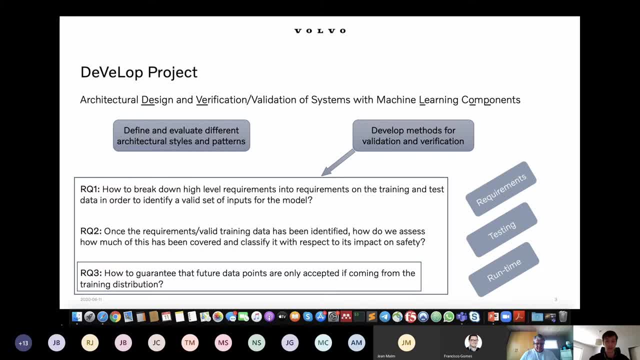 We need to define and evaluate different architectural styles and patterns. And also verificational part. We want to develop methods for validation and verification of systems and machine learning components. And in this- oops, sorry, in this project, in this presentation, I will focus on the validation part. 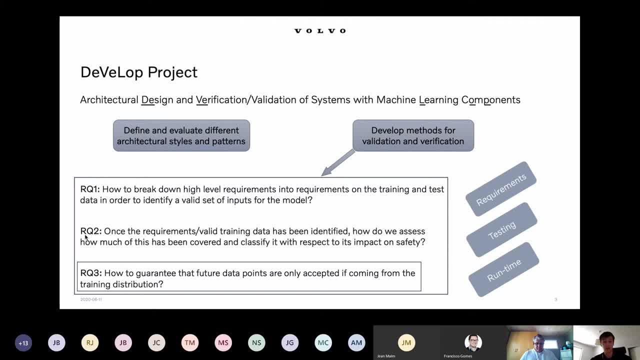 We can outline three research questions here. First first research question relates to requirements. It's we can formulate it as a how we can break down high level requirements on the training and test data sets in order to to be sure that we covered all the valid set of inputs. 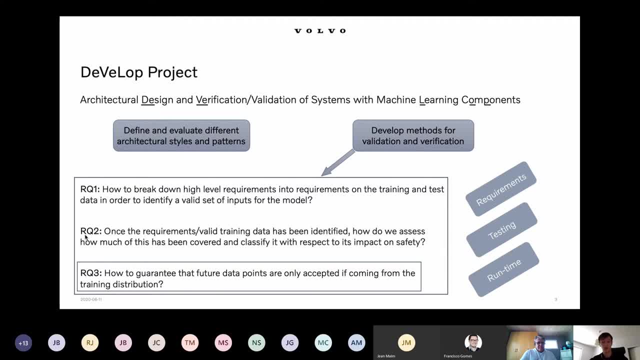 The second research question relates to the testing phase. We want to use this break down requirements and validate and evaluate how much of this data we covered during the training and testing. And then the last one is for runtime, when we want to make sure that during the run time in the self-driving car, for example, we we allow only the input data which is coming from the distribution similar to the, to those which was used during the training, and to reject those data which coming out of from out of training data distribution. 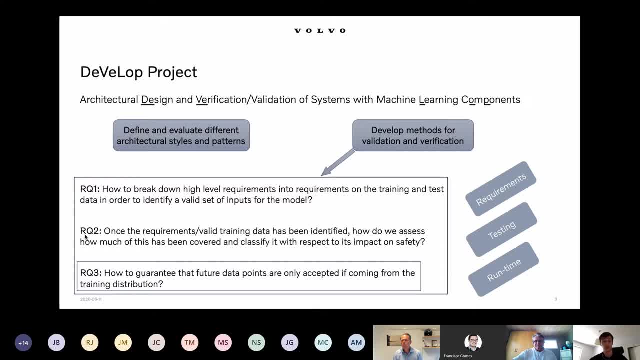 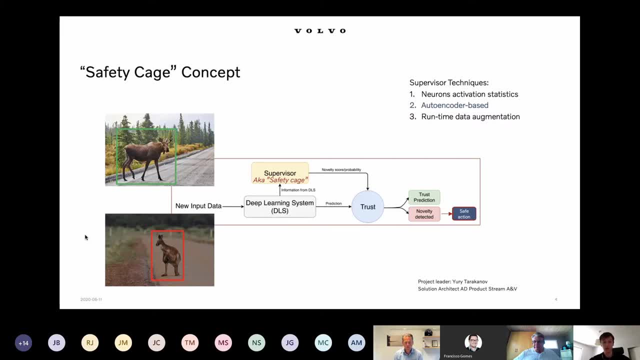 And this is exactly what what this anomaly detection project is About. here we comes to the concept of the safety cage. This safety cage allows to actually implement this anomaly detection in the self-driving car for some deep learning system or machine learning system inside. 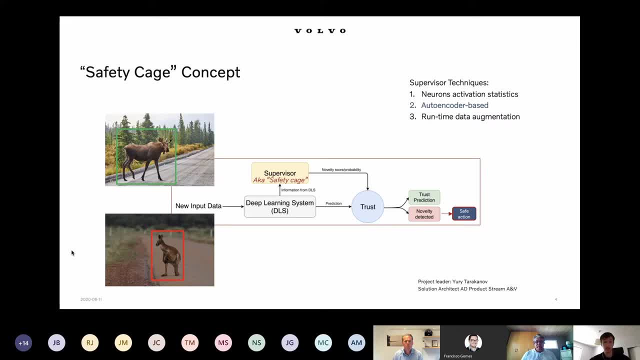 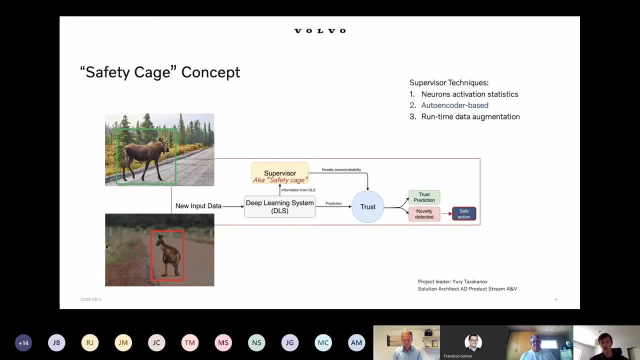 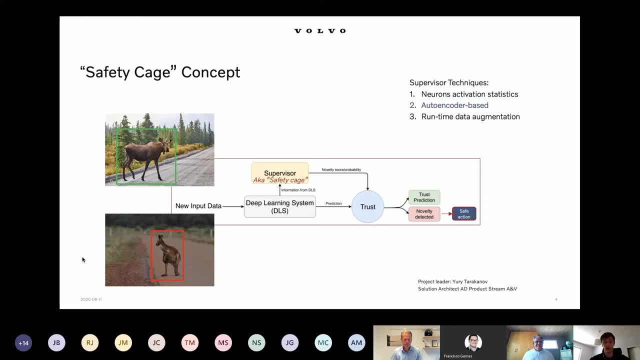 And for this we actually need this object detection algorithm to have the code of this, Okay, Okay. The second one which I will talk about is autoencoder-based anomaly detection. Here, for this technique, we implement a separate algorithm which is based on autoencoder. 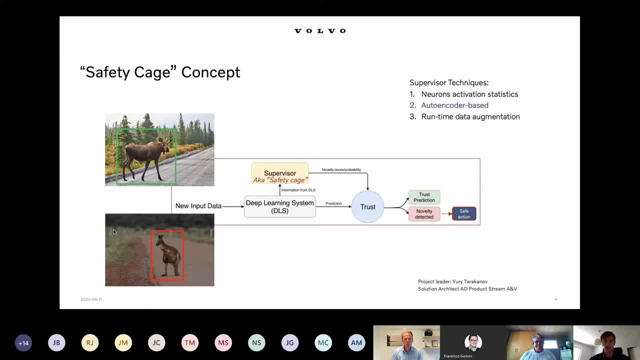 and we run it in parallel with object detection algorithm here and it output the anomaly score of the input data. For this we don't need to have this object detection algorithm here, we just can train it separately, this autoencoder. The third option is to use runtime data augmentation. 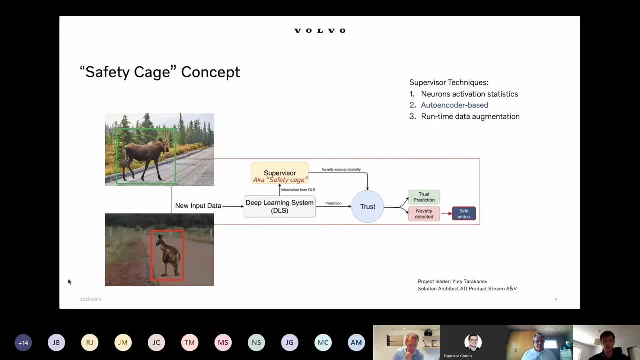 and it's actually related to manipulation of the input data During the perception phase and inference phase. when we detect objects, we manipulate input data several times and augment it and see how- for different modifications, how the object detection algorithm behaves, and based on this, 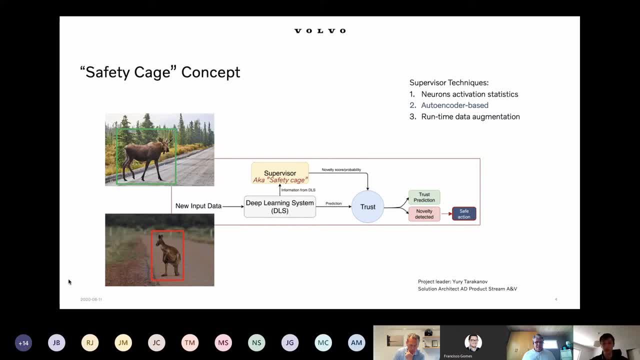 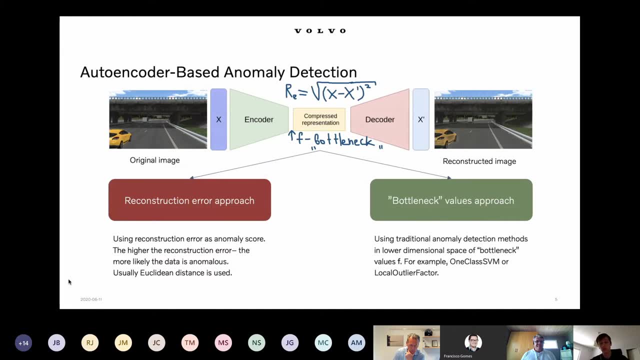 we either trust or reject the input data. In this project I'm talking about autoencoder-based. What is the autoencoder? Autoencoder is a special type of neural networks. It actually has the input and the output- the same, and the main goal of the autoencoder. 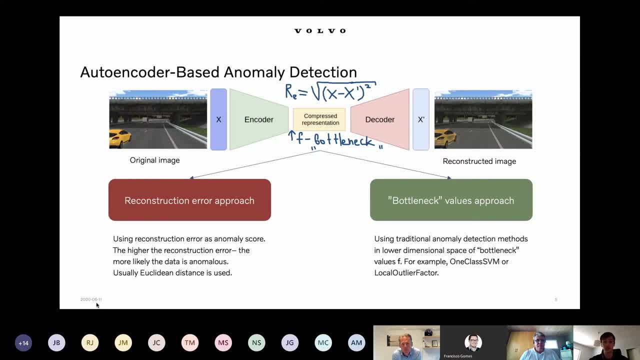 was solving the task of dimensionality reduction. It's mainly used for dimensionality reduction, just like the dimensionality reduction of images. It basically have the so-called bottleneck in the middle in between all this autoencoder, and it has encoder and decoder part. 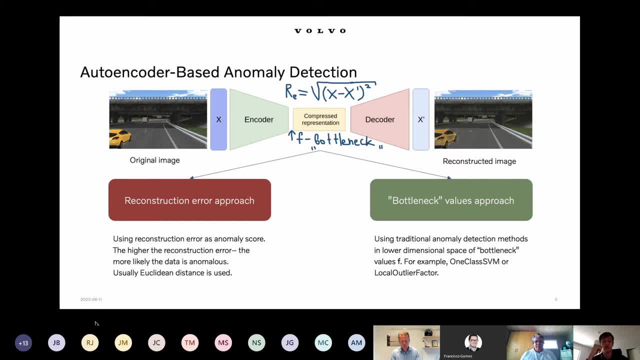 We have also two different approaches for an autoencoder-based anomaly detection. The first one is using the construction error approach. When we calculate the reconstruction error between the input and the output, image error is a anomaly score as an indicator how much our output data deviates from. 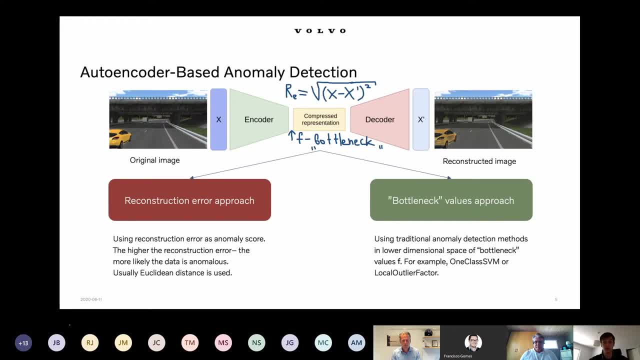 the input data. because the assumption is that if we train autoencoder only on the normal data, without using anomaly data, then we will be able to reconstruct the normal data during the runtime very good, so the reconstruction error will be low. and if we feed the anomaly data into the autoencoder during the runtime, then 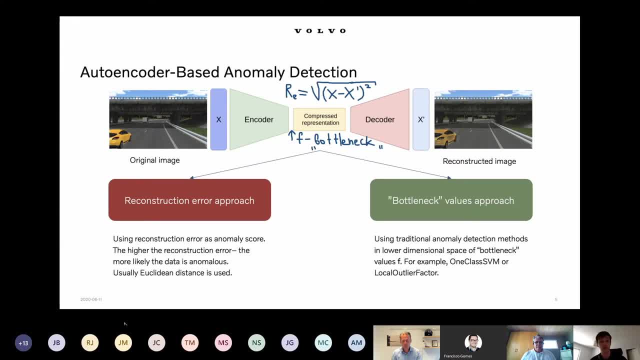 it will not be able to reconstruct this data very, very good and we will have a higher reconstruction error. so we can use it as anomaly score. and the second approach is to use bottleneck values in the middle of the autoencoder, because the assumption is that autoencoder learn some important information inside of 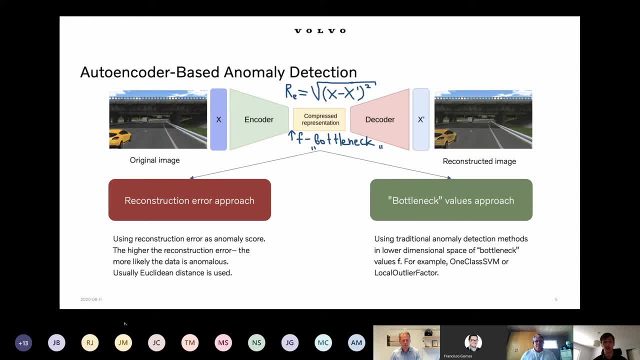 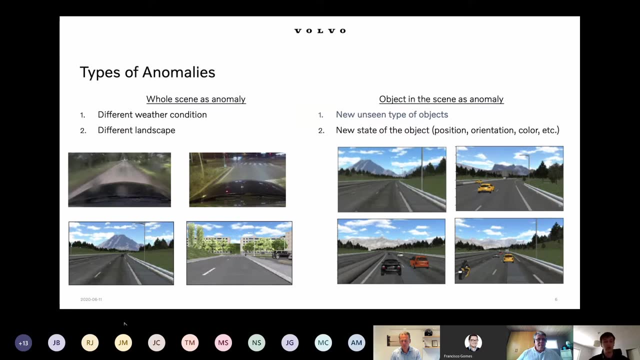 inside of it and we can basically use it bottleneck values. it's basically a feature vector and we can use traditional anomaly detection algorithms on these bottleneck values. so next important thing is to mention about different types of anomalies which can be monitored during the cell jarring run. there are two types. the first one on the 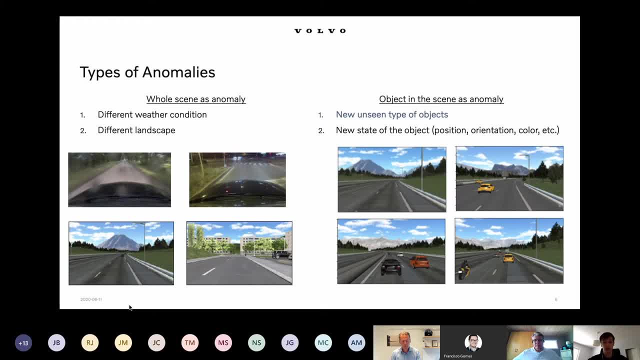 left. you can see it's a. when we use a whole scene as anomaly, meaning that it can be either different weather conditions- for example, it can be rain or fog or night- we can say that this is anomaly, or it can be in different landscape, for example, when we 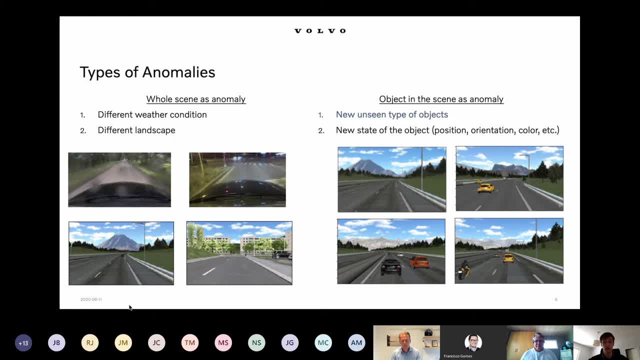 trained our object detection algorithm on a highway and we want to use it in the city traffic scenario. it's also will be anomaly for the object detection algorithm. and on the right you can see a much more difficult case, which is when we, when we say that some, some particular type of object is anomaly, which will, which was? 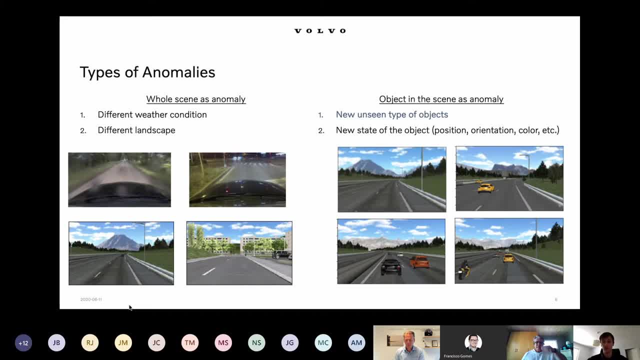 unseen during the training phase because, for example, here it b machine learning model or obligation algorithm was trained on empty highways without cars. and once we fit into this, obligation is an image with cars. it will not understand. want to what? what to do with this car? it will classify. 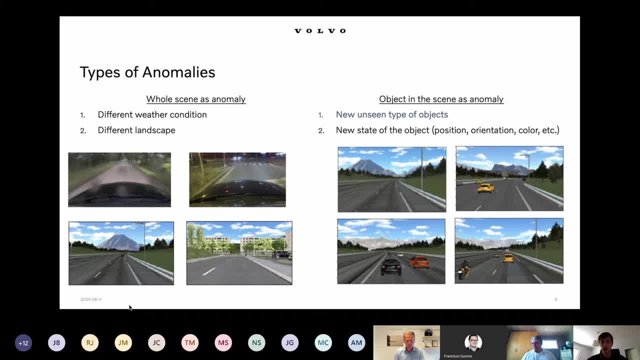 it wrongly, or another case when we trained it on cars. but we want to also detect pedestrians. it also pedestrians will be also anomalous in our case because it will output some some wrong decision because it hasn't seen this pedestrians during during the training phase. it also can be. 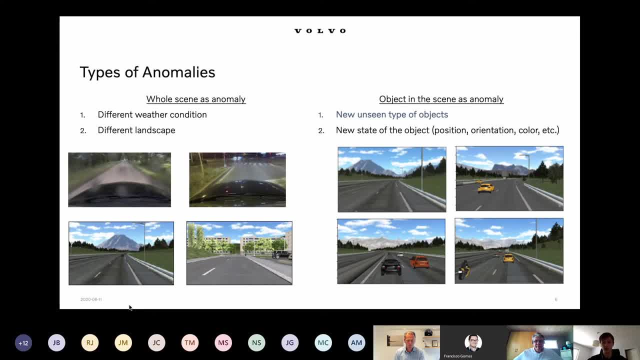 some new state of the object, for example position orientation, for example pedestrian upside down. it will be also anomaly if it was not presented in the training set and what we also observed during preliminary research that this. these are all of the existing anomaly detection algorithms. they are very dependent on the color. 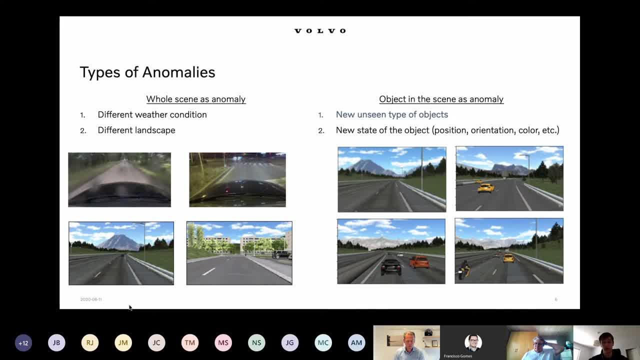 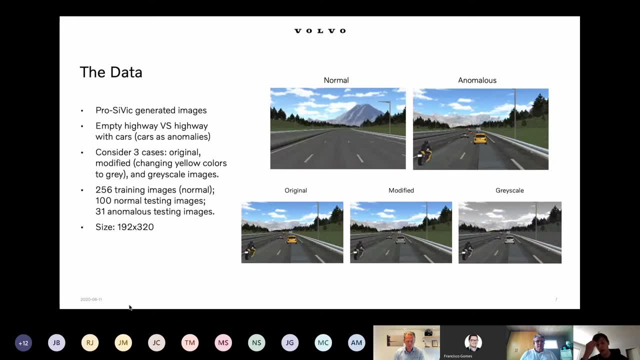 information on the pixel brightness values presented in the images and i will show you later what. what is it? yeah, here. so uh, we wanted, we wanted to compare these two described earlier approach, i know, for anomaly detection based on auto encoders, mainly reconstruction error approach and bottleneck values. we wanted to estimate the performance of anomaly detection and also we 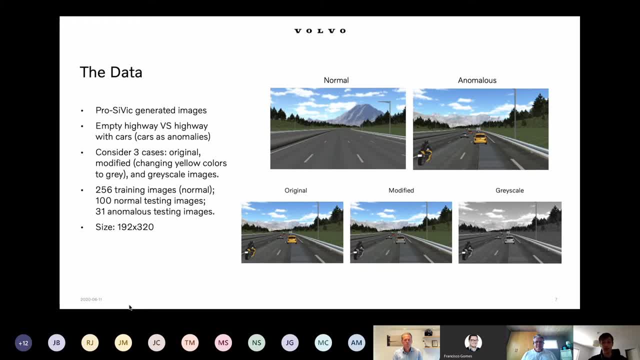 wanted to compare them between each other, and for this we use the generated data from pro civic. of course, the ultimate goal is to apply our anomaly detection algorithm on real data, but we are currently on the experimental phase and during this phase we can manipulate the colors and objects easily on in the generation. 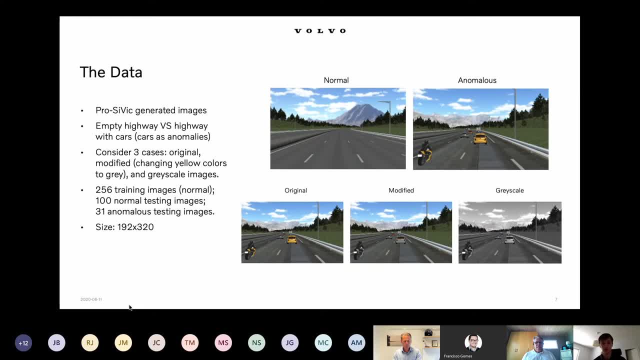 in the generation engine and then we are going to also already apply it on the real data. so for now it's only generated data. so here you can see that we consider the case when we have a anomalies, when we have cars as anomalies, so we consider normal scenario when we have an empty. 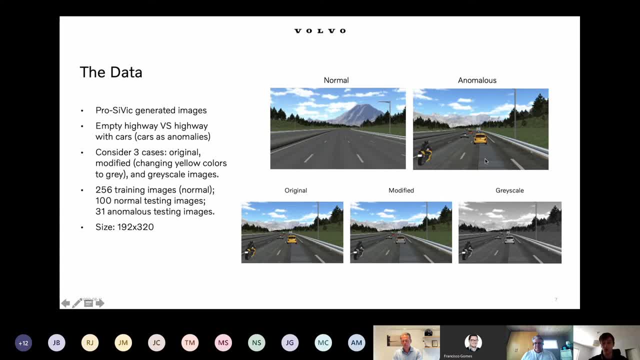 road and once we have a car here or motorcycle or truck, we consider this image as an as anomalous image. it's very simplified case, but it's also is a descriptive. there is also very descriptive and we consider three different scenarios when we take original images with all the colors. the second one is more tricky, we change. 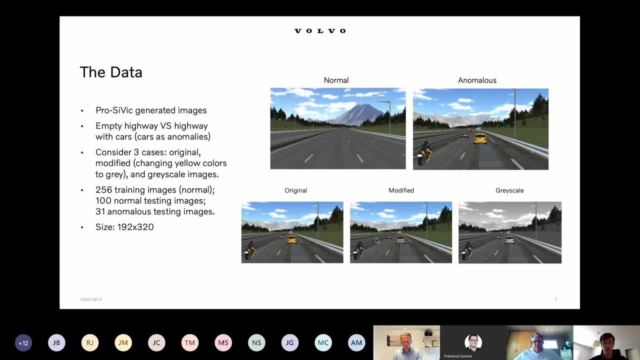 the all yellow, bright, bright yellow colors and the images to the gray to see how, how it will influence the results of anomaly detection. and also, here we consider the case when we remove the color information completely from the images. we trans, uh, we transform it to great scaled images and we had a 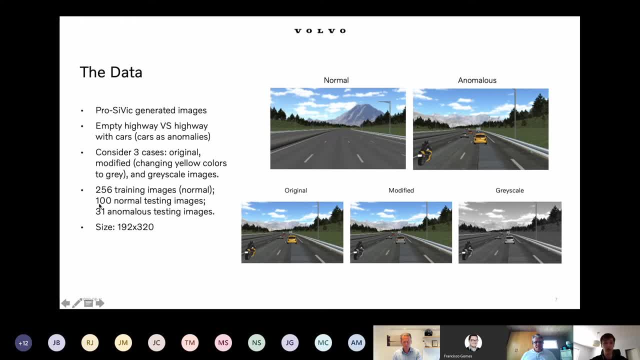 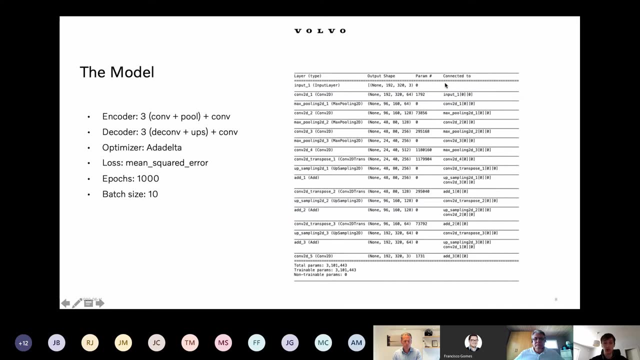 256 training images for training our auto encoder model and we had 100 normal and 31 anomalous uh images for testing our anomaly detection algorithm. uh, a little bit about the model itself. so here is our actual auto encoder uh. it consists of the encoder part and decoder part. encoder ends here. so we had we have a three. 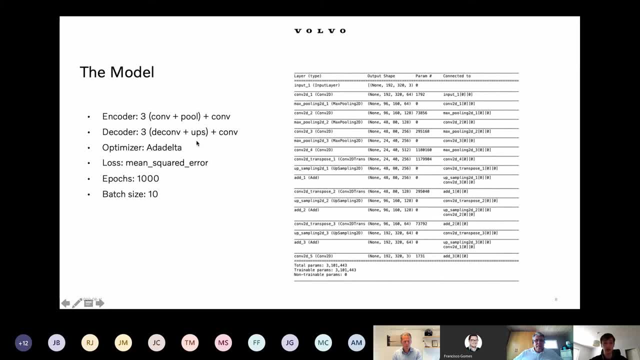 plus pooling layers and in the decoder part we have three deconvolutional and up sampling layers. so we implemented it in keras, a simple model. we trained it with optimizer idle. other delta we used mean squared loss function, trained for 1000 epochs and use batch size equals 10.. 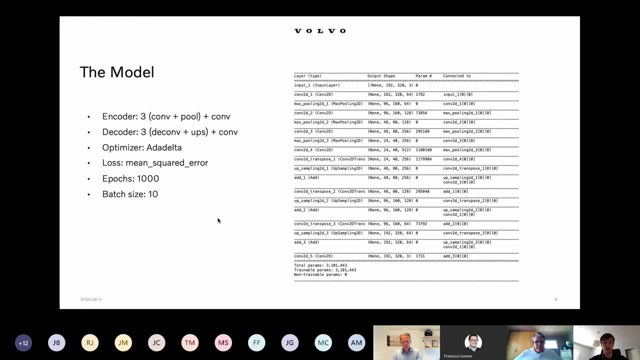 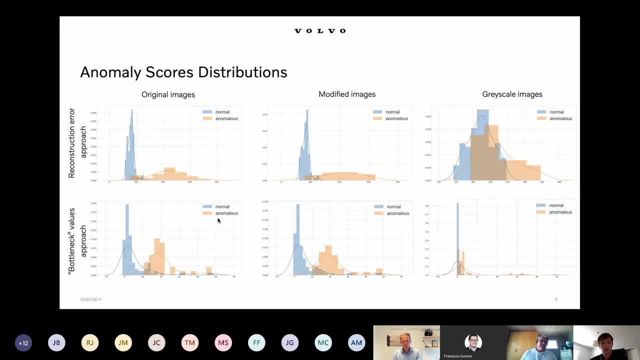 so, yeah, a little bit technical information. it's supported for reproducibility of our results. and then we actually. the first step was that we have visualized our anomaly scores, returned by our autoencoder based anomaly detection algorithms, and here we put on these plots for every case, for original images, modified images and grayscale images, and for 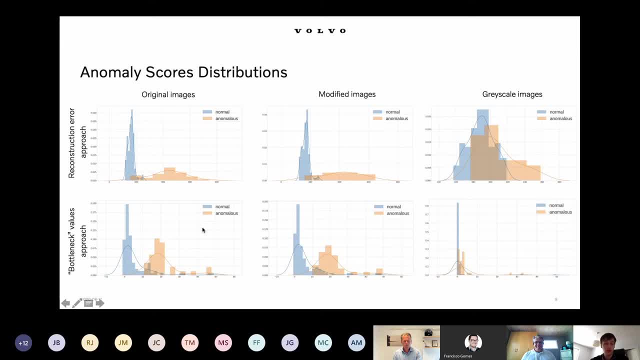 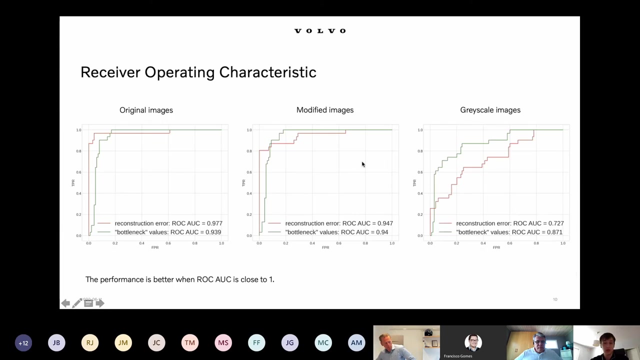 different approach. our construction error and bottleneck values lower row and we can see that for when we use the original images we have. we had a very clear separation- not very, we had some intersection here, but these two groups of normal and anomalous images were we could separate with some threshold here. once, oops, once we change the color of the 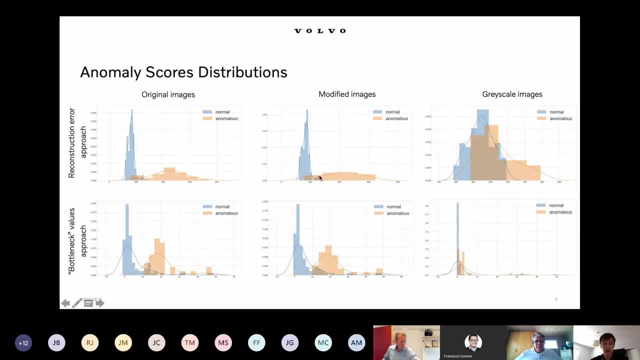 yellow cars to the gray. this peak was a little bit smooth and the intersection became bigger, and when we used grail scaled images we were mixing up two sets of images: normal and anomalous images- completely or more or less completely. so these two distributions of anomaly scores for 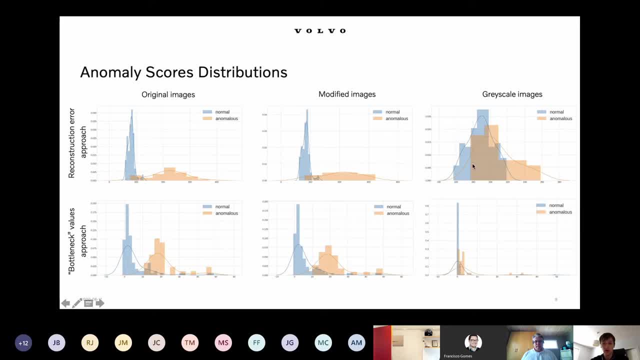 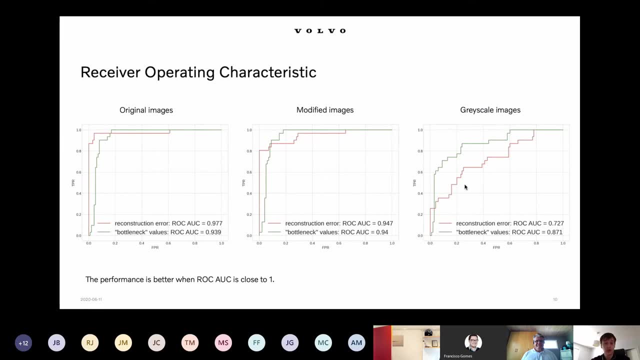 normal and anomalous images. uh, we will put it on each other and in order to compare the results numerically, we have considered this anomaly detection task as a binary classification problem. so we use this anomaly detection as a binary classificator, saying that, outputting that either is that anomaly or not, and from here we can see that putting a different 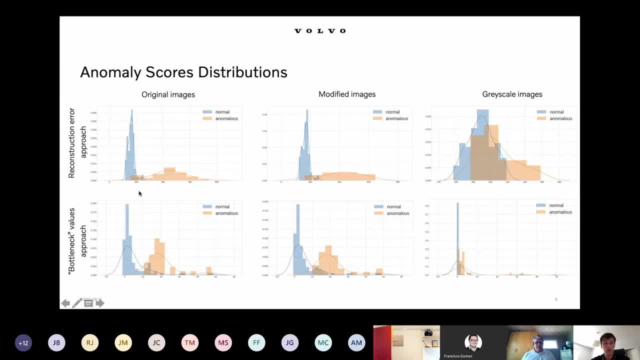 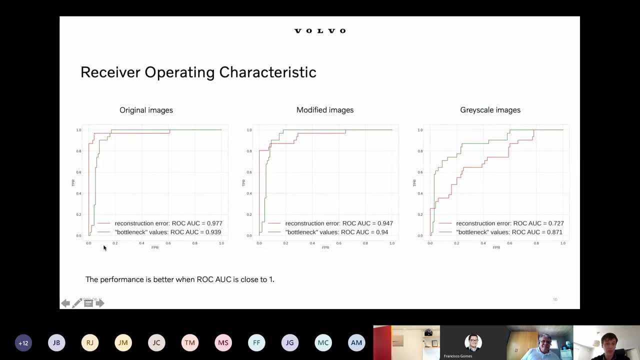 threshold on the anomaly score. we can put it here or here: using a different threshold, we can obtain different true positive and false positive rates, and we actually can plot these true positive rates and false positive rates for different threshold values of anomaly detection scores and this thing will- uh, it's called receive operating characteristic curve. 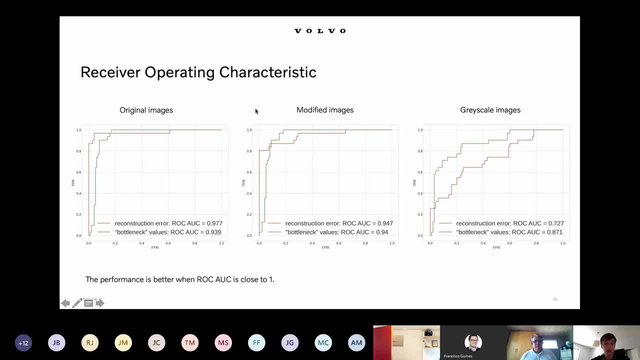 it's usually used for for assessing the performance of binary classification problem and also we can calculate the area under this curve and it will correspond to the overall performance of anomaly detection. and this area under this curve can vary from zero to one, and once it's closer to one, 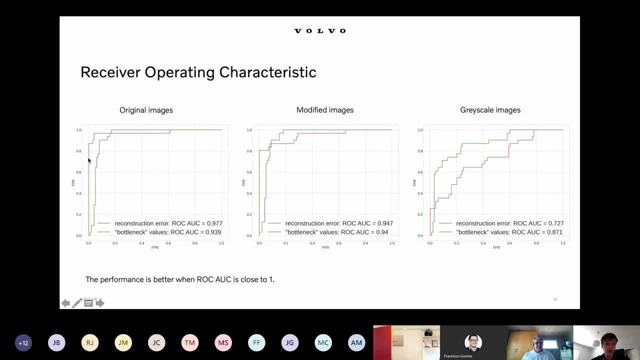 the performance of anomaly detection is higher because we want to have this curve going to the left top corner, closer to the left top corner, where we have 100 true positive rate and zero false positive rate. and looking at the left picture, uh, this, this is the case when we used original images. 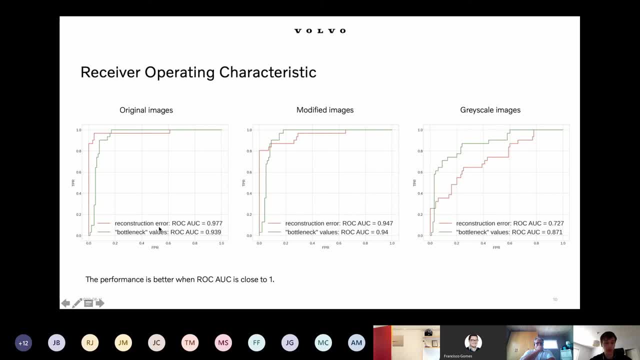 with all the colors and they see that the reconstruction error approach outperforms a little bit the bottleneck values approach. uh, according to rocaux, area under curve, when we change the color of the yellow cars to the gray cars and motorcycles and trucks, we actually see that reconstruction error approach performance decreases a little bit. 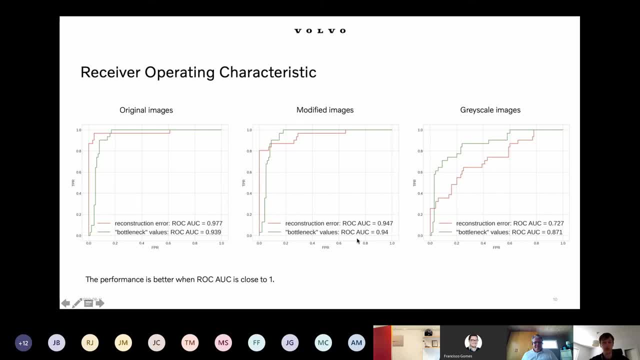 up to 0.947, while the bottleneck values wasn't affected by this change. changing on the color and also once we have a grail scale images on the right, the, we see that uh bottleneck uh values approach still shows some more or less good performance. uh, with uh rocaux score equals 0.871, but the reconstruction error approach almost approaching. 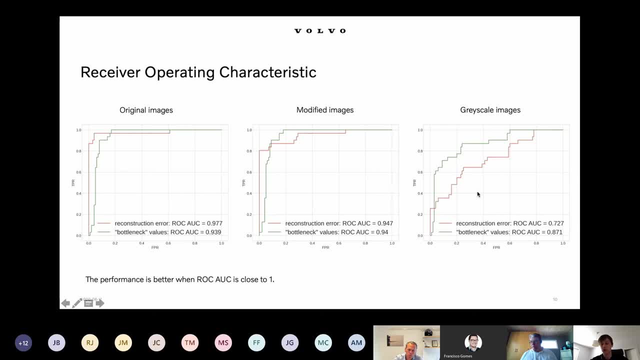 a random guessing line which is approaching 0.5 rocaux score, where we have a random guest lecture, and from this we can conclude that this bottleneck values approach- it wasn't affected by the modification of the color information, but the reconstruction error approach was influenced a lot, so we're changing the color. 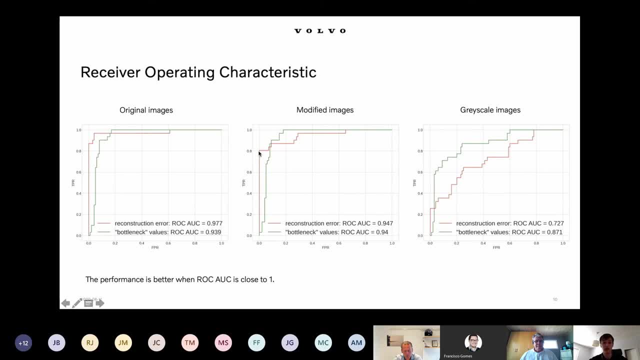 only only yellow cars to the gray and it's we already see significantly significant drop in the performance of anomaly detection for reconstruction or approach and for the grail scale images also. it's decreases even more and, what is also important here, if we look at the point where we have a true 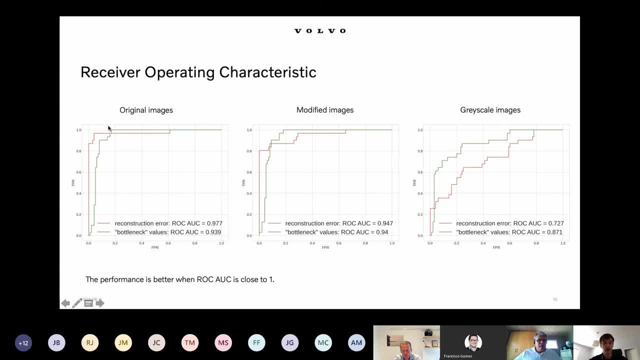 positive rate equals 100 percent. uh, this is the most important point from uh from the perspective of cell driving context, because we want to have this true positive rate always to be 100. we want to detect all the anomalies but at the same time we want to maintain a relatively low false positive. 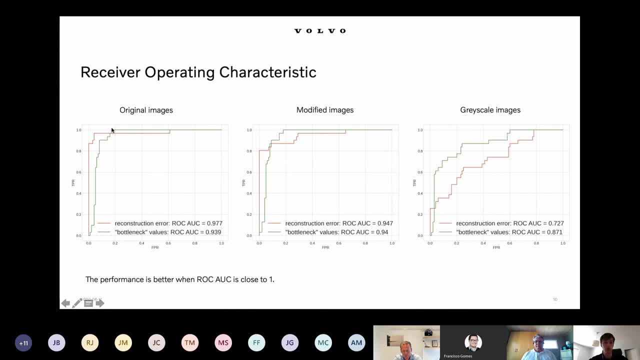 rate, which is the case for a bottleneck values approach, because we can see from the pictures it allows to have a. for example, in the case of original images on the left plot we can see that we have a 100 true positive rate, uh, at this point and we have less than 0.24 positive rate of anomaly. 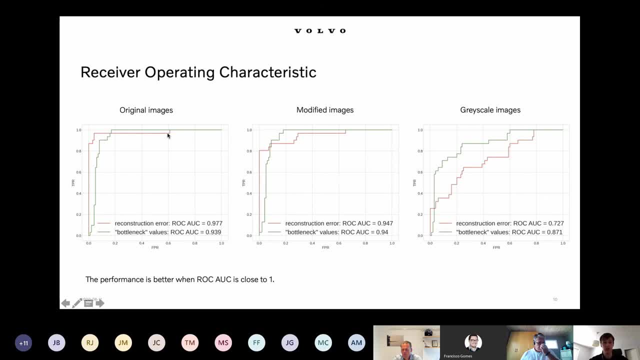 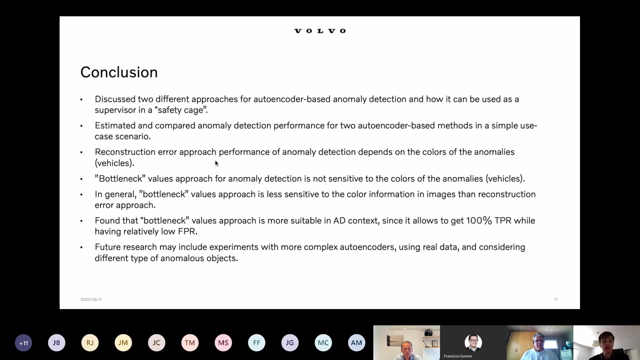 detection, while for a construction approach it's not the case. when we have a 100 true positive rate for the construction error approach, we we actually texture detect more than 60 percent of false-positive anomalies, which is not good. To conclude, I've presented: 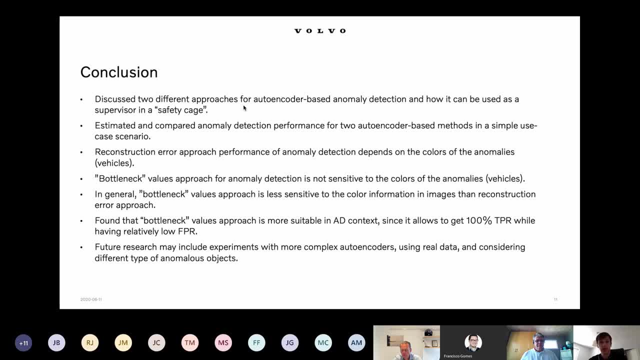 two different approach of autoencoder-based anomaly detection on a high level. I discussed how it is used in the context of a safety cage, because it's important to understand how it can be. how can it be used in the actual self-driving car architecture? 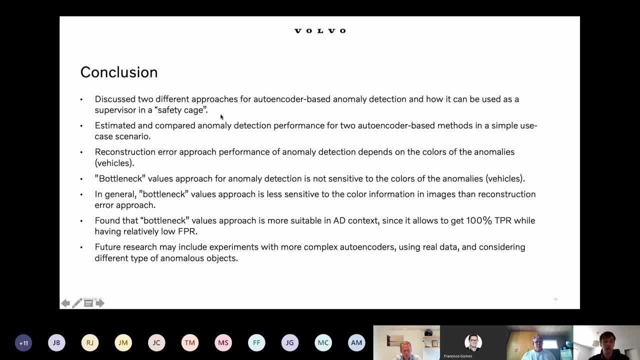 and it's actually acts as a safety cage. So we detect anomalies and we actually trust or reject the output of our deep learning model. Also, we estimated and compared the performance of two autoencoder-based methods using a simple use case scenarios on generated data. 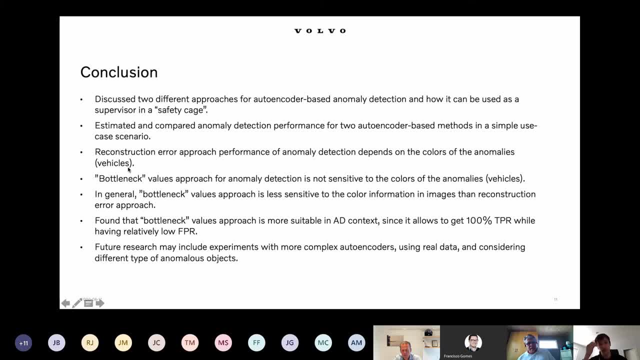 We also showed that reconstruction error approach performance- it's affected a lot by the color manipulation on the images, while the bottleneck approach wasn't affected so much, At least when we change the yellow cars to the gray color of our cars, But in general also. 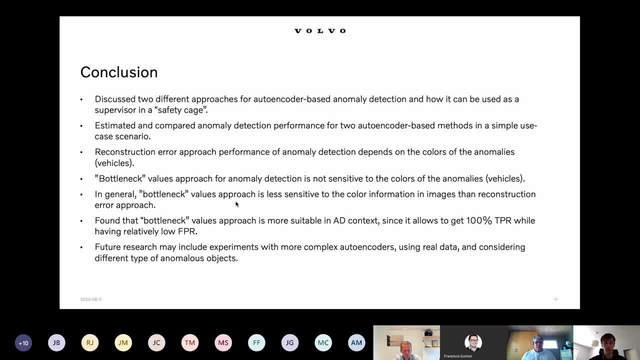 when we used grail-scaled images, bottleneck wireless approach also showed the high performance of anomaly detection. This bottleneck wireless approach also allows us to maintain a 100 percent true positive rate with less than 0.2 false positive rate, which is also good in the context of autonomous driving. 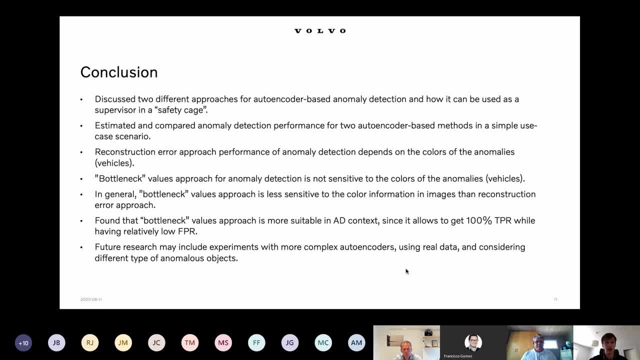 These things. they can be correlated with the results of Smile2 project, which was finished a recent time ago And there AFTROS also investigated this problem of anomaly detection and safety cages, And they were focused more on the different types of anomalies rather than objects. 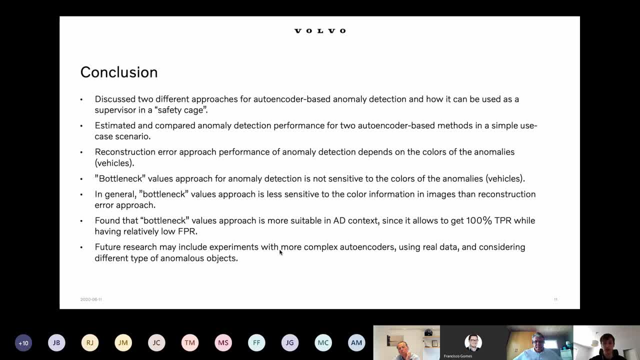 They were focused on the weather conditions and landscape scenarios, But they also think that when we have object as anomalies, it's more difficult And we also need to work in this direction, And the future research may have to include the experiments with more complex autoencoder architecture. 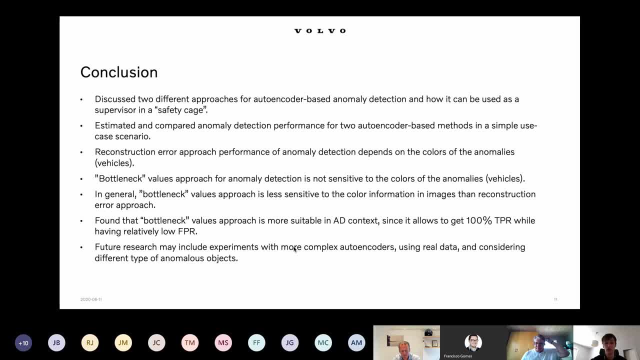 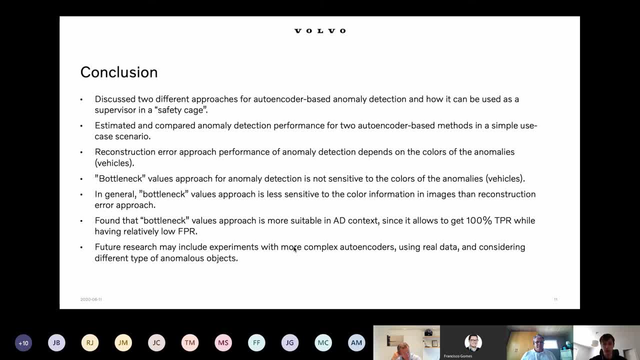